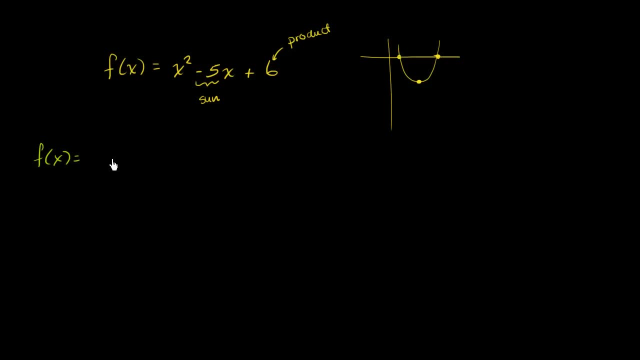 And so let me write it this way: We could write f of x as being equal to x minus 2 times x minus 3.. Now, how does this help us find the 0's? Well, in what situations is this right-hand expression? 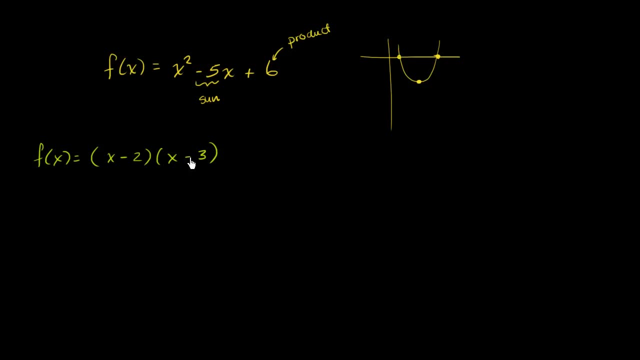 is this expression on the right-hand going to be equal to 0?? Well, it's the product of these two expressions. If either one of these is equal to 0, 0 times, anything is 0.. 0 times anything else is 0.. 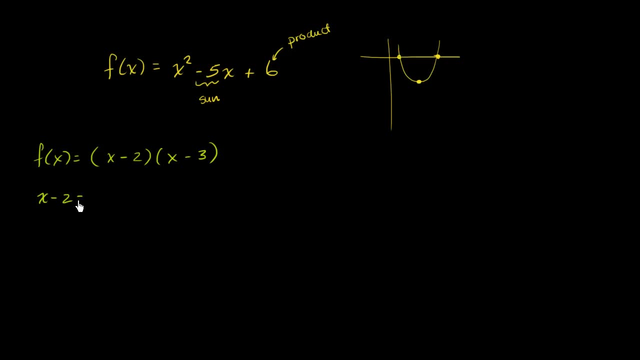 So this whole thing is going to be 0 if x minus 2 is equal to 0 or x minus 3 is equal to 0. Add 2 to both sides of this equation. you get x is equal to 2 or x is equal to 3.. 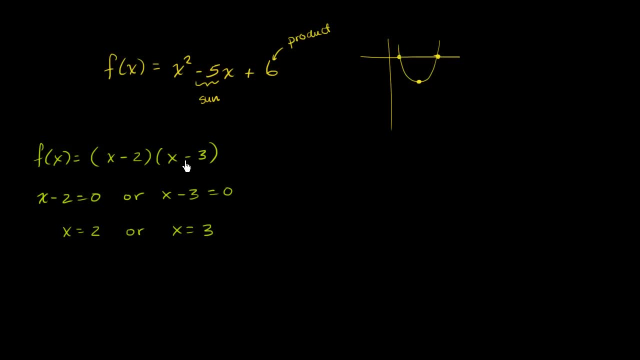 So those are the two 0's For this function. I guess you could say, And we could already think about it a little bit in terms of graphing it. So, if we wanted to, so let's try to graph this thing. 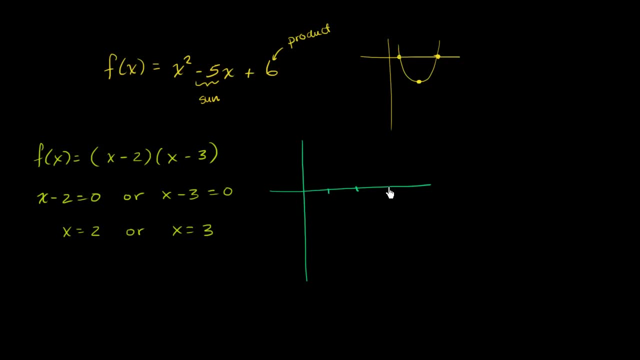 So this is x equals 1.. This is x equals 2.. This is x equals 3, right over there. So that's our x-axis. That you could say is, our y is equal to f of x-axis And we're seeing that we intersect. 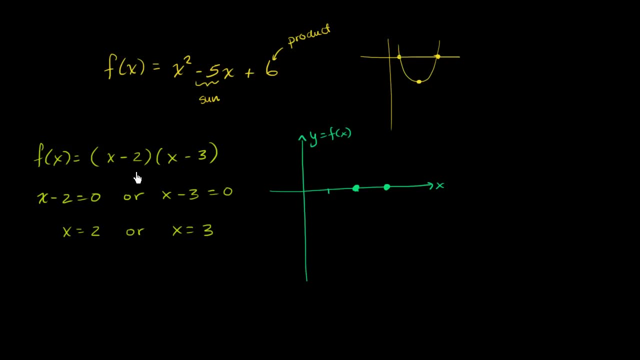 both here Here and here. When x is equal to 2, this f of x is equal to 0.. When x is equal to 3, f of x is equal to 0. And you could substitute either of these values into the original expression. 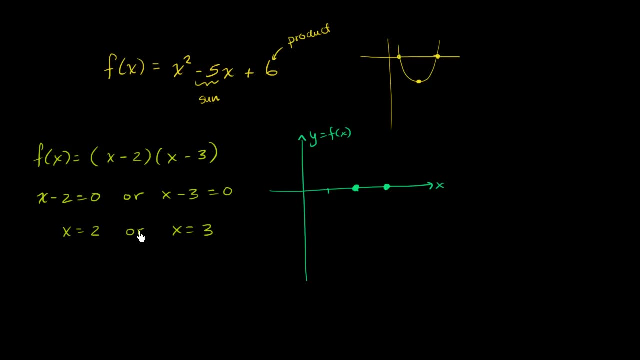 And you'll see it's going to get you to 0, because that is the same thing as that. Now, what about the vertex? What form could we write this original thing in order to pick out the vertex? Well, we're already a little familiar. 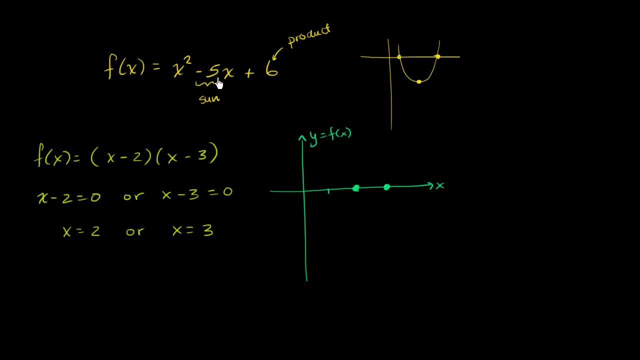 with completing the square, And when you put it in that form, or when you complete the square with this expression, that seems to be a pretty good way of thinking about what the minimum value of this function is. So let's just do that right over here. 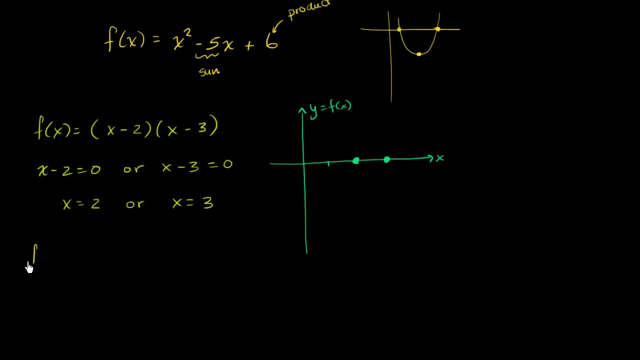 So I'm just going to rewrite it So we get: f of x is equal to x squared minus 5x, And I'm just going to throw the plus 6 right over here And I'm giving myself some real estate, because what I need to do, what I want to think about doing, 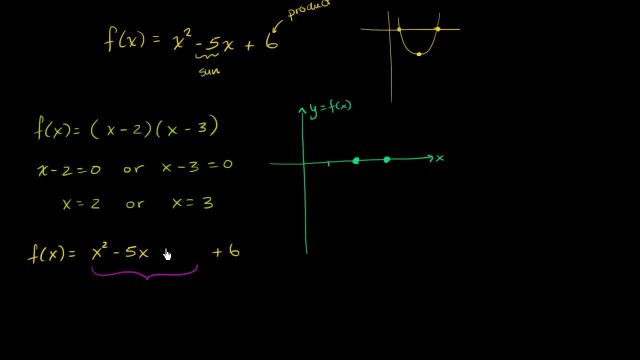 is adding and subtracting the same value. So I'm going to add it here and I'm going to subtract it there, And I can do that, because then I've just done it. I've added 0.. I haven't changed the value of this right-hand side. 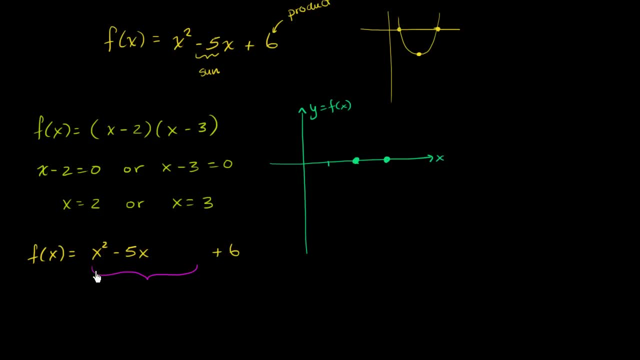 But I want to do that so that this part that I've underlined, or in this magenta color, so that this part right over here is a perfect square, And we've done this multiple times when we've completed the square. I encourage you to watch those videos. 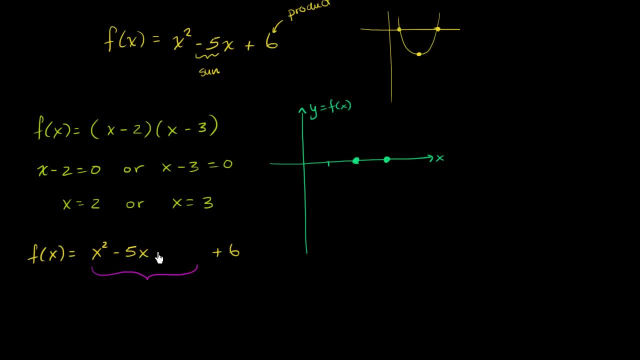 if you need a little bit of a review on it, But the general idea is this is going to be a perfect square. If we take this coefficient right over here, we take negative 5, we take half of that which is negative 5 halves and we square it. 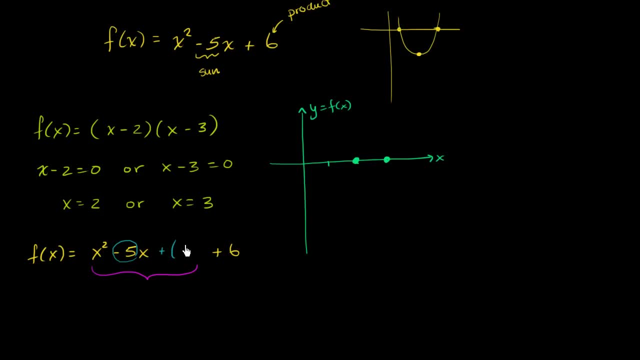 So we could write this as plus negative. What's negative? 5 halves squared. So I could write this: negative 5 halves squared. Well, if we square a negative number, it's just going to be a positive, So it's going to be the same thing as 5 halves squared. 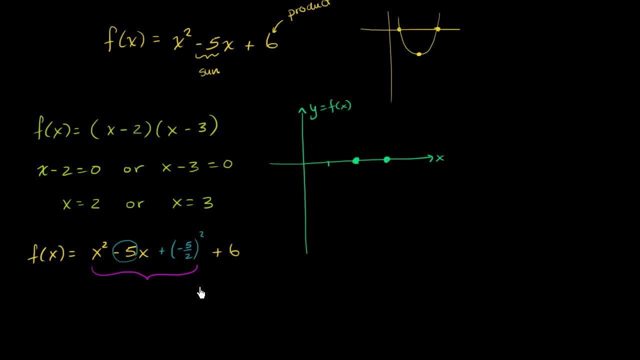 5 squared is 25.. 2 squared is 4.. So this is going to be plus 25 over 4.. Now, once again, if we want this equality to be true, we either have to add the same thing to both sides, or if we're 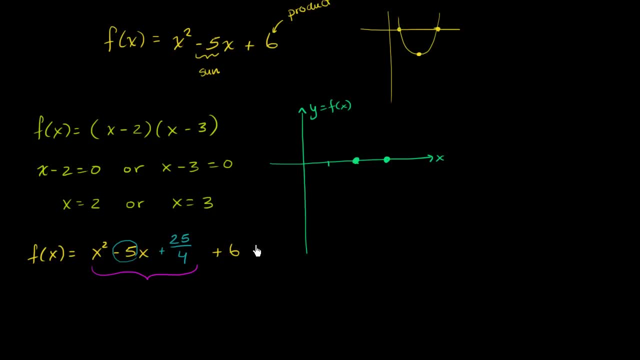 just operating on one side. if we added it to that side, we could just subtract it from that side, And we haven't changed the total value on that side. So we added 25 over 4, and we subtracted 25 over 4.. 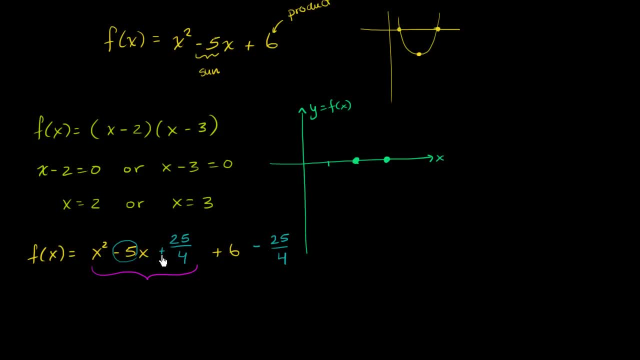 So what does this part right over here, what does this become the part that I've underlined in magenta? Well, the whole reason why we engineered it in this way is so that this could be x minus 5 over 2 squared. 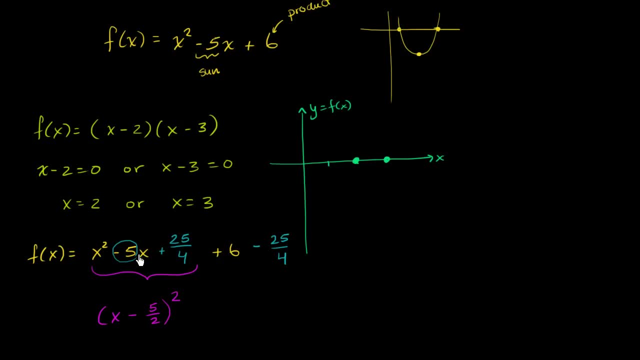 And I encourage you to verify this- And we go into more detail. We're going to go into more detail. We're going to go into more detail. We're going to go into more detail about why, taking half the coefficient here and then squaring it, adding it there, 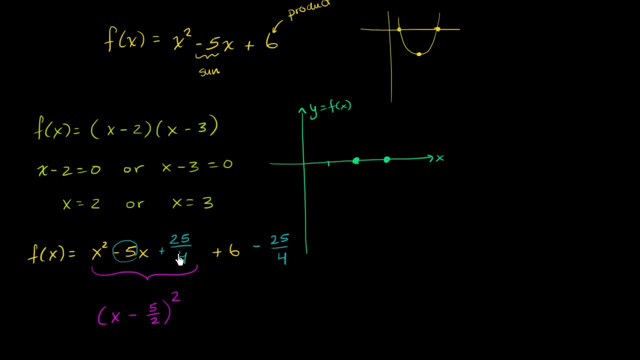 and then subtracting there why that works. We do that in the completing the square videos, But these two things you can verify that they are equivalent. So that's that part, And now we just have to simplify: 6 minus 25 over 4.. 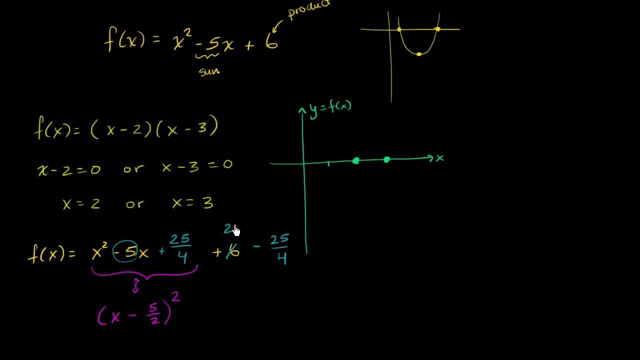 So 6 could be rewritten as 24 over 4.. 24 over 4 minus 25 over 4 is negative 1 fourth, So minus 1 fourth, Just like that. So we've rewritten our original function as f of x. 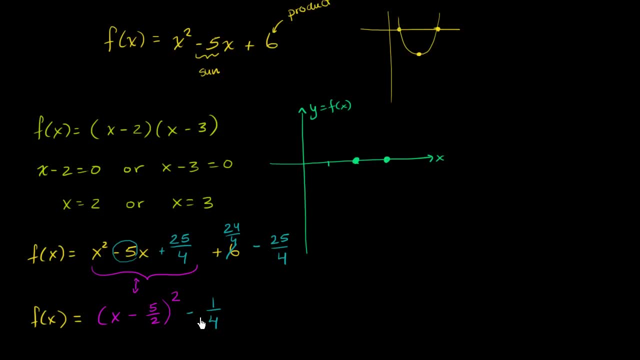 is equal to x minus 5 halves squared minus 1 fourth. Now, why is this form interesting? Well, one way to think about it is: this part is always going to be non-negative. The minimum value of this part in magenta is going to be 0.. 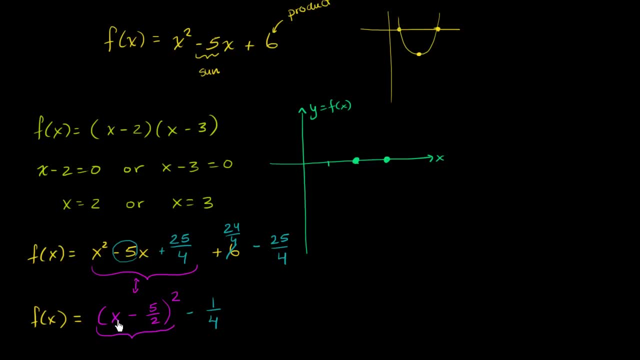 Why? Because we're squaring this thing. If you're taking something like this and we're just dealing with real numbers and you're squaring it, you're not going to be able to get a negative value At the minimum value. this is going to be 0.. 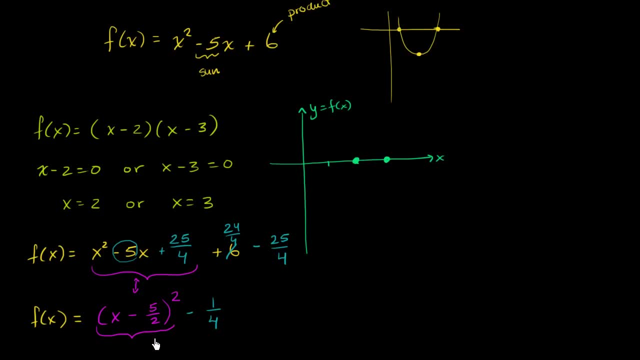 And then it obviously could be positive values as well. So if we want to think about when does this thing hit its minimum value? Well, it hits its minimum value when you're squaring 0.. And when are you squaring 0?? 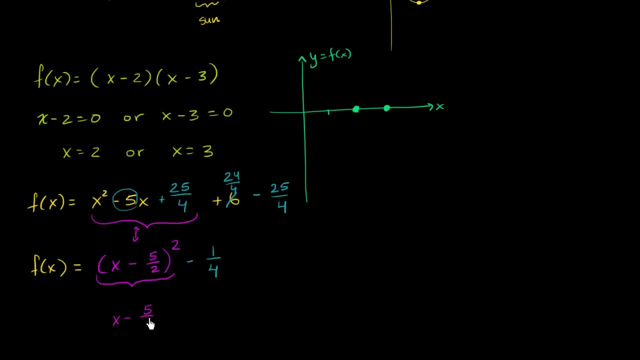 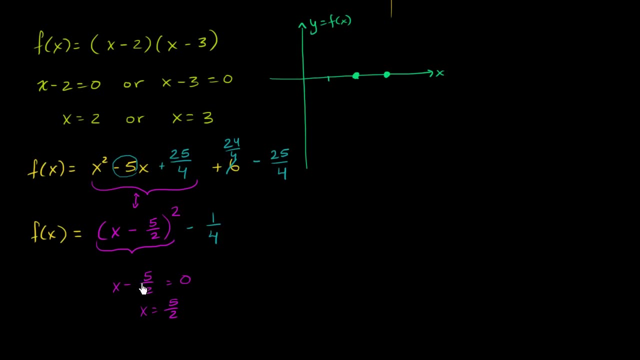 Well, you're squaring 0 when x minus 5 halves is equal to 0. Or when x is equal to 5 halves, if you just want to add 5 halves to both sides of that Equation, So this thing hits its minimum value. 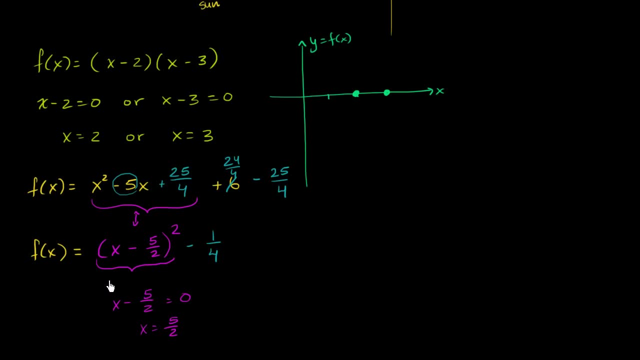 when x is equal to 5 halves. And then what is y or what is f of x when x is equal to 5 halves? And once again, you could use any of those forms to evaluate 5 halves, but it's really easy in this form. 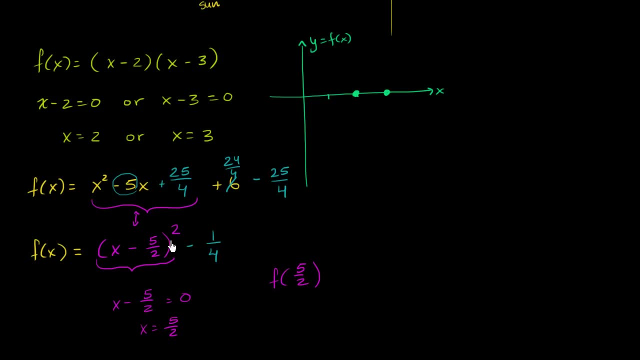 When x is equal to 5 halves, this term right over here becomes 0, 0 squared 0.. You're just left with negative 1 fourth. So another way to think about it is: our vertex is at the point. So we could say: our vertex is at the point, x equals 5 halves. 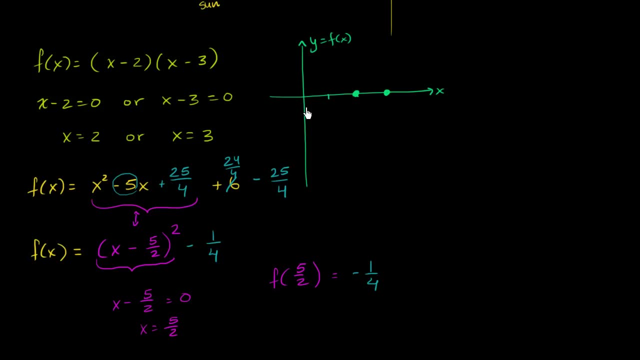 y equals negative 1 fourth. So x equals 5 halves. That's the same thing as 2 and 1 half. So x equals 5 halves And y is equal to negative 1 fourth. So if that is negative 1, 1 fourth. 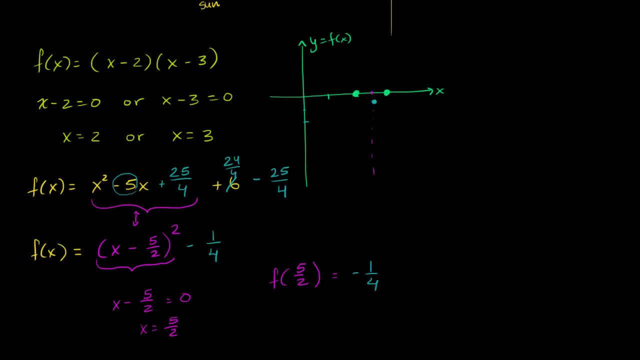 would be something like that, So that right over there is a vertex. That is the point. Let me make it clear. That's the point. 5, halves comma negative 1. fourth, And what's cool is we've just used this form.